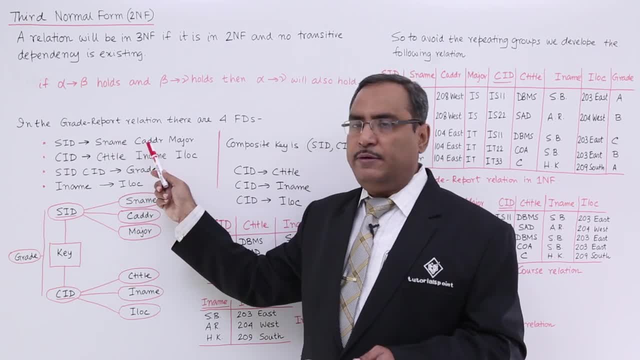 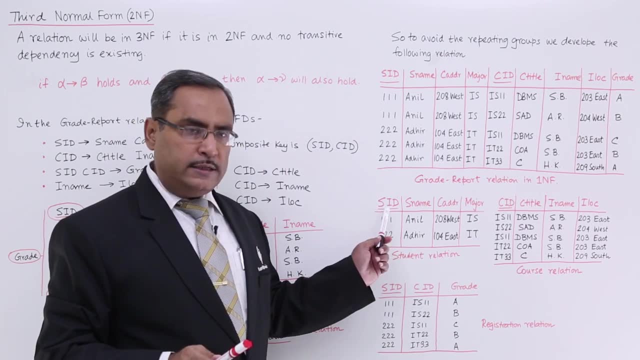 one was: student ID determines student name, campus address and major. Depending on that, we develop this student name, campus address and major. So we have a student name, campus address and major, keinen an element which means a student, student, student ID, student identity, student name or any students name or however. 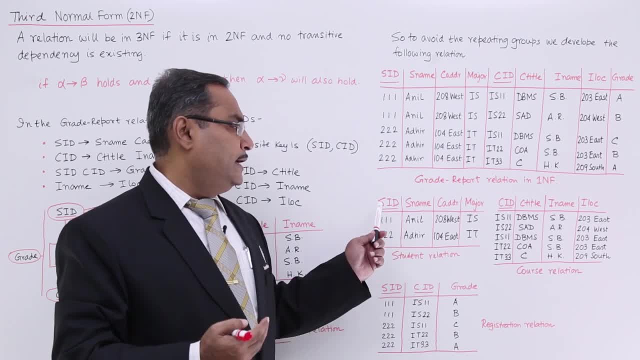 same thing can be used for треть party, or a third party to determine which student identityNG is legendary or not. So the legal requirement 교육 이동 되고 이 명령이 관건인 동기자 real nameique all these types of 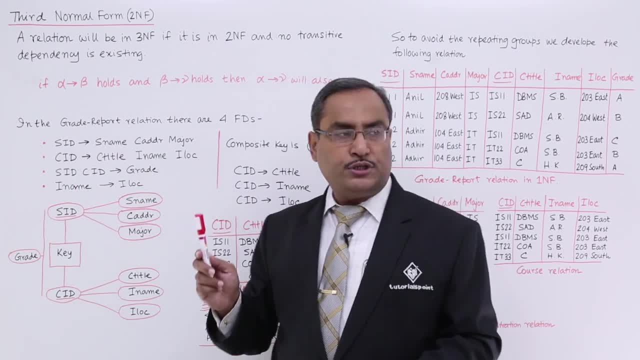 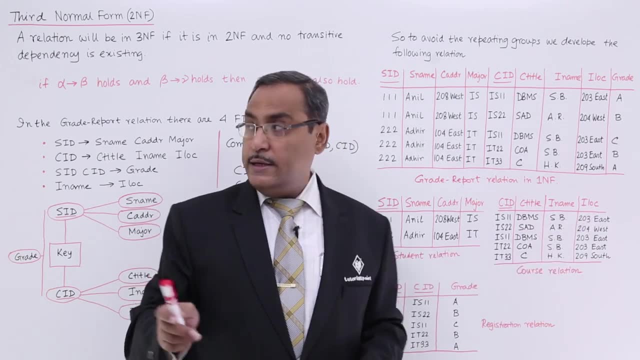 each of them took full role in determining exactly the general level of difficulty for each student identity. Finally, în order to obtain wouldn t have 자 가고, And this determinant, That is, the student ID which is falling on the left hand side of the functional dependency, is a prime attribute or the primary key. Second, was course ID determines course title. 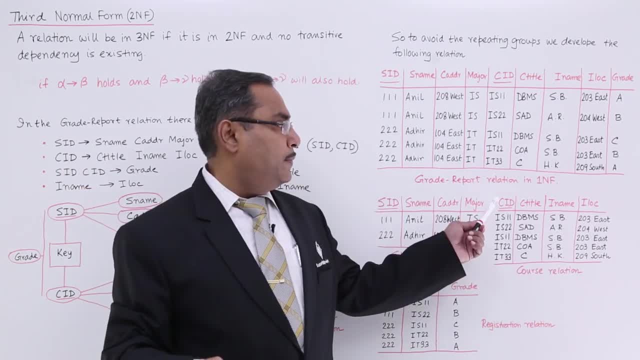 instructor names and instructor location. So we will be going for course ID determines course title, instructor's name and instructor's location. Here the determinant determine the degree of the dominant. that is, our course id will be the primary key and other are the non-prime attributes. 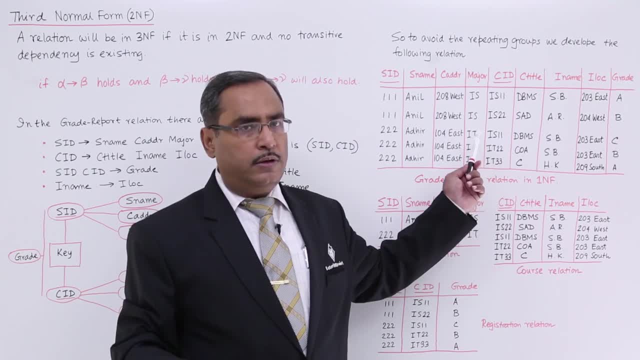 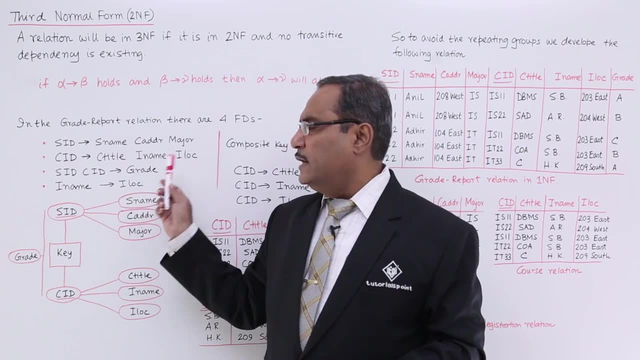 In this way the data got extracted from the mother table mother relation which was in 1NF. Next one was student id course id determines grade. So student id course id determines grade. So this particular relation is formed. 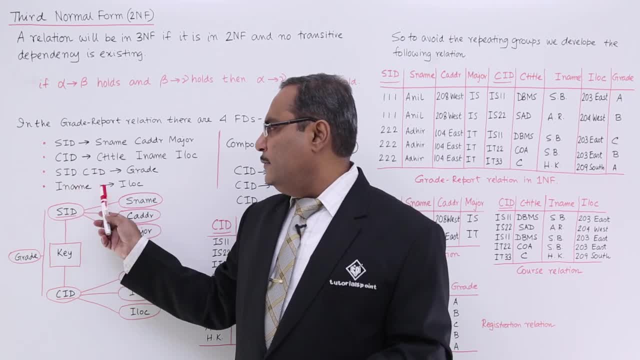 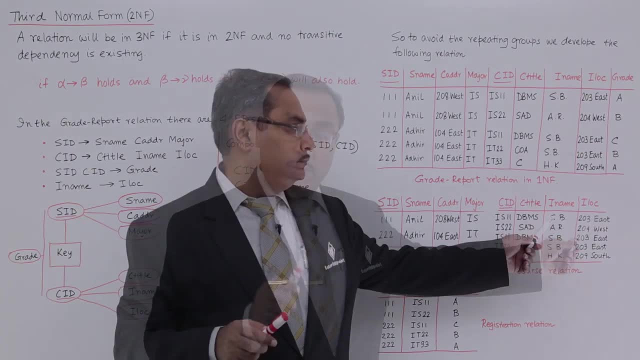 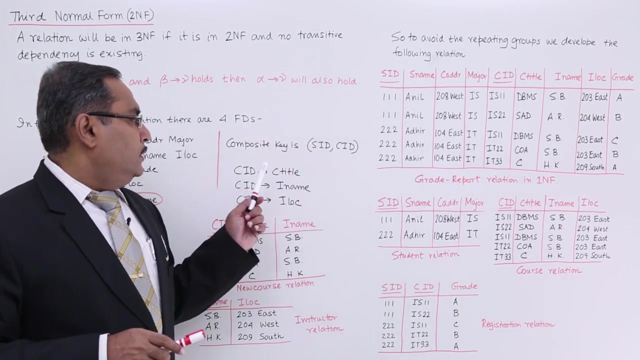 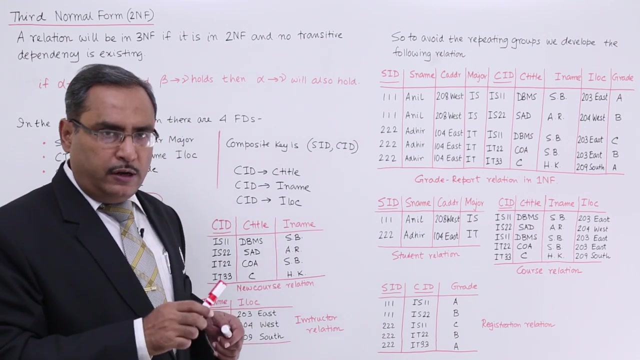 The last functional dependency was: instructor name determines instructor location. So here we are having instructor name determines instructor location. So here we are getting the flavor of transitive dependency. Why See course id determines course title, course instructor's name and instructor's location. So that particular functional dependency on that we have applied. 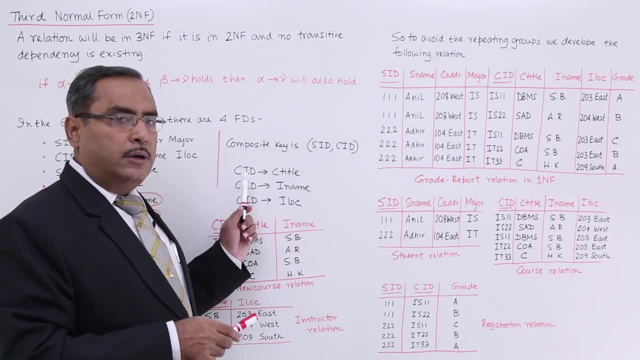 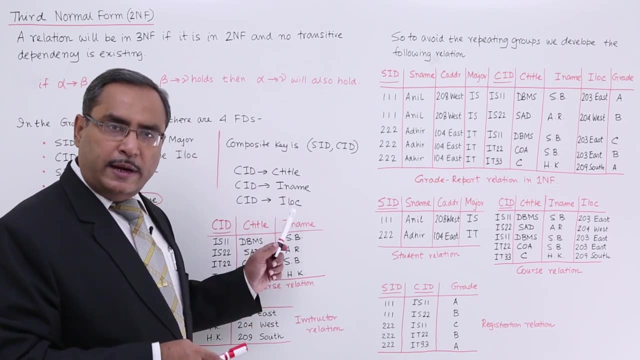 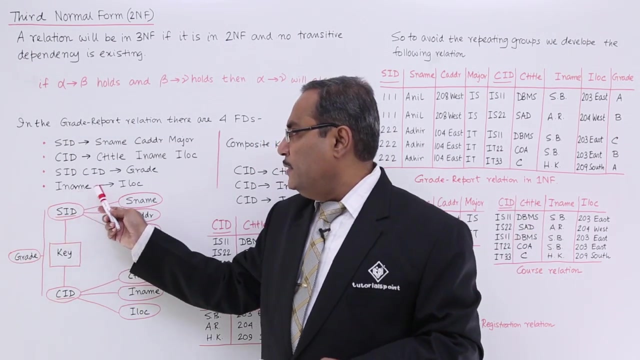 the decomposition rule. So I am reaching with: course id determines course title. course id determines instructor's name. So we are having course id determines instructor location. Also we are having instructor name determines instructor location, So course id determines instructor's name and instructor's. 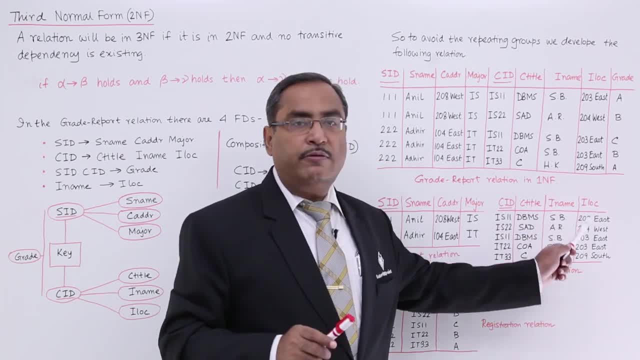 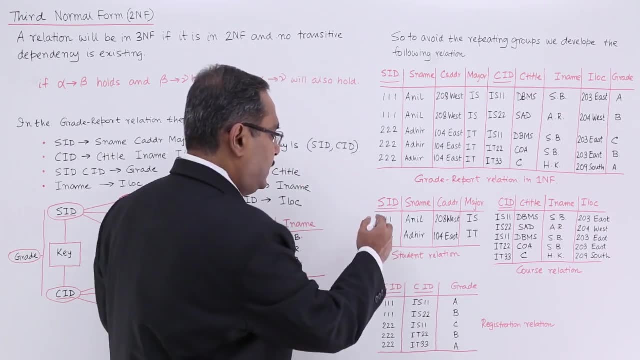 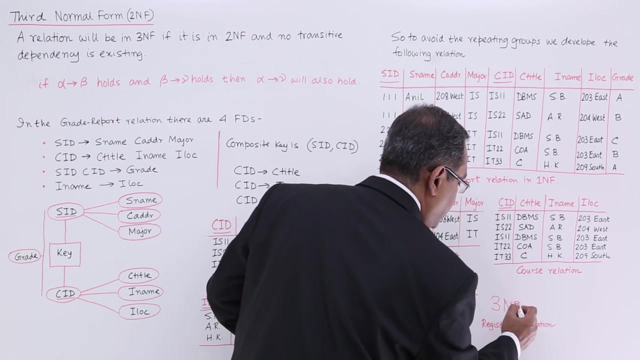 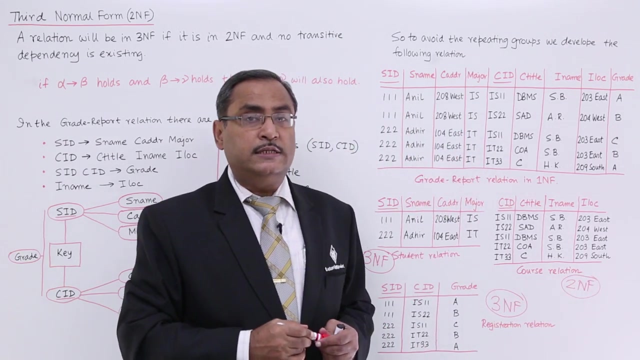 name is determining instructor's location. So there is a transitive dependency here. So this particular relation is not in 3NF. So this relation is in 3NF. This relation is also in 3NF, but this relation is only in 2NF. why? because this relation have in the. 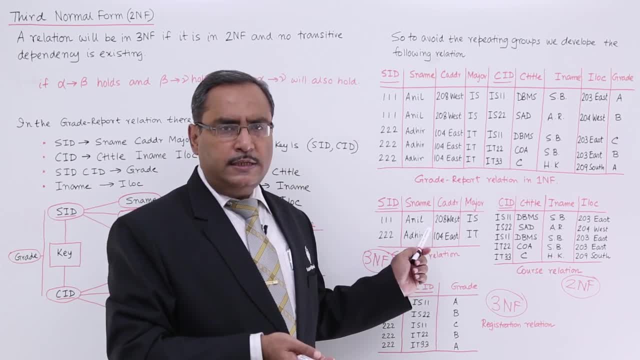 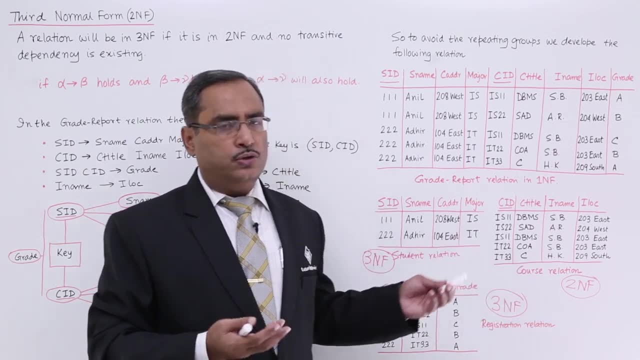 transitive dependency here. Only one functional dependency is there. So that is the very common one, that the prime attributes will determine all other non-prime attribute. So there is no question of having any transitive dependency. Same thing is logically stressed. So this witness relation is declared. So this is showing that this is now 2NF and which is also 2NF. So this rosenthal relation is found in 2NF, This is be found in 2NF. So this relation has been kind of propagated. 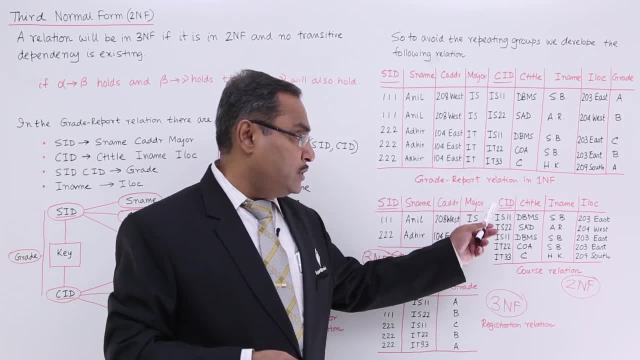 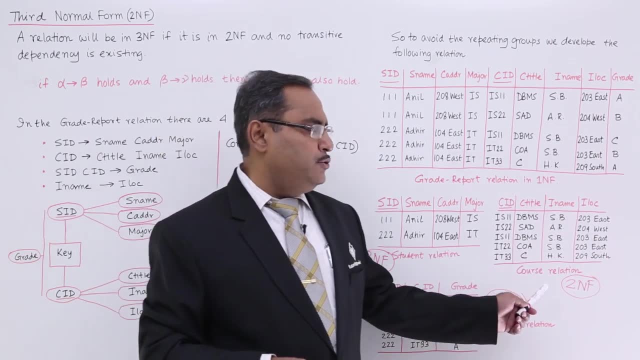 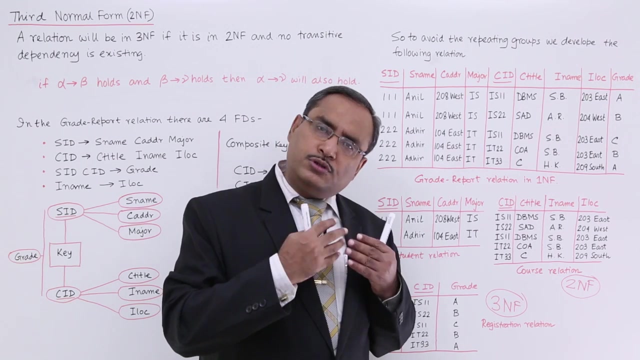 logic is true for here also. but here we are having: course id determines instructor's name and instructor names determines instructor location. so you might be asking me: it is in 2nf, it is not in 3nf that we got. but what is the difficulty in that case? difficulty means those: 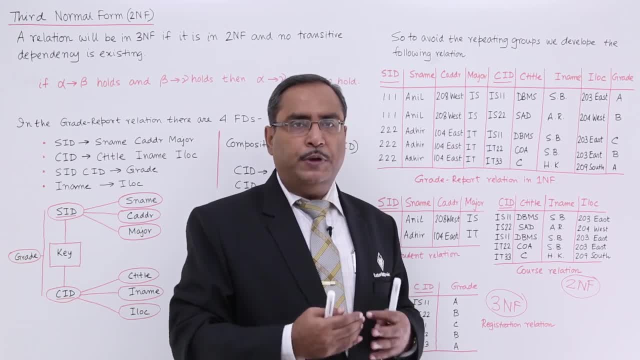 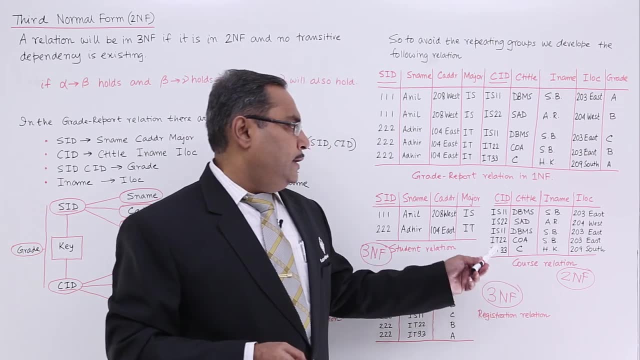 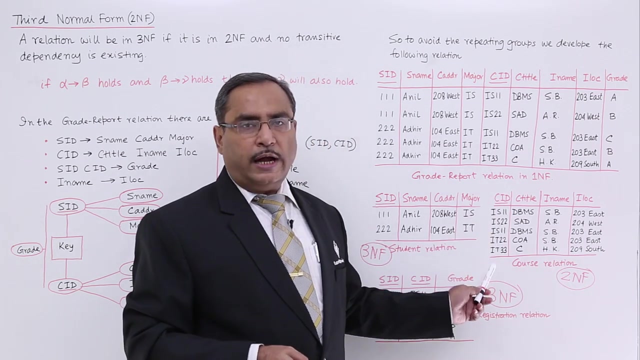 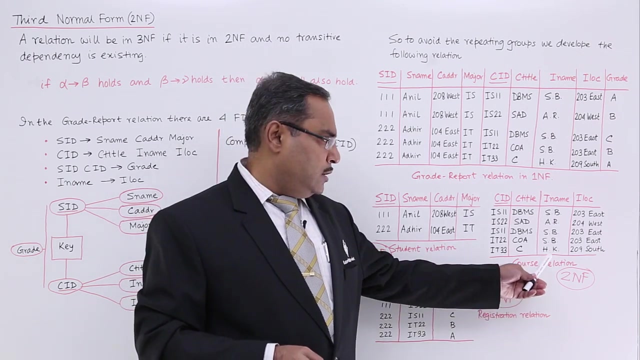 three same anomalies: insertion, deletion and updation anomalies. on this relation, we cannot perform insert, delete or update operation. i am just showing you this is my course id, so i cannot insert any record. i cannot insert any record, keeping this course id null. let us suppose one new instructor has joined to this particular university with a certain name and also the 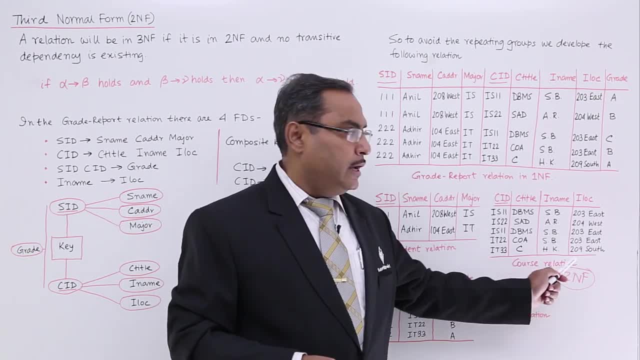 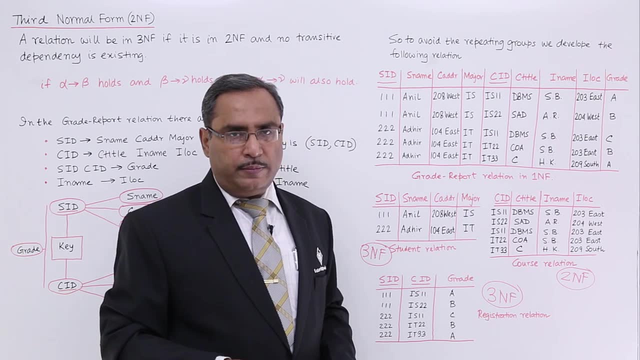 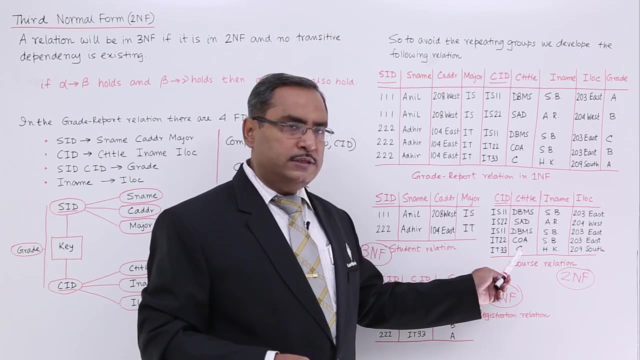 accommodation address. we know i cannot make an entry until and unless that instructor has got one course assigned to him or her. so that is the insertion anomaly, deletion anomaly- deletion anomaly means there is only one course, so that is one course. is there the course on c and h? k said used to take this particular. 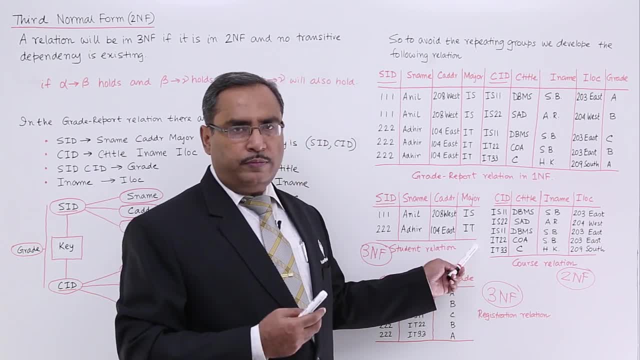 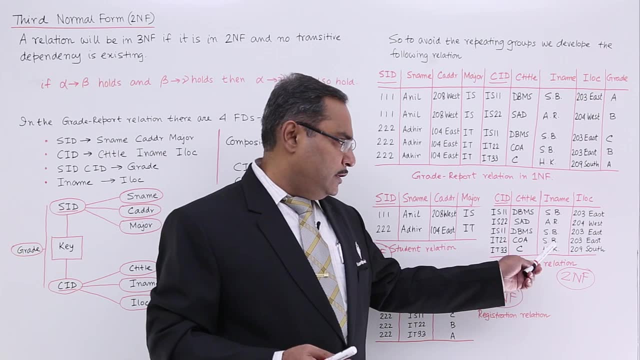 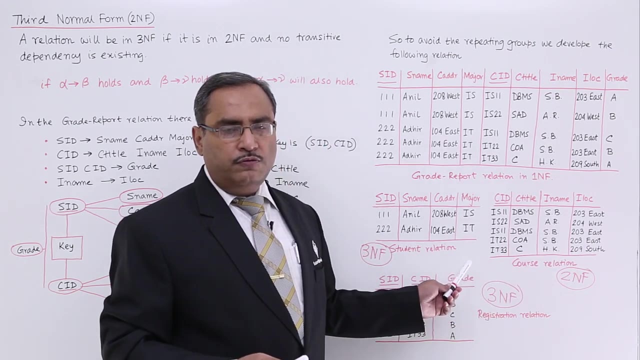 classes. so now university has withdrawn this course from the from the syllabus, so this tuple is getting deleted, along with the information regarding this new faculty is getting deleted, so this particular faculty record will get deleted if the university withdraw this particular course from the syllabus. so that is our deletion anomaly. let us 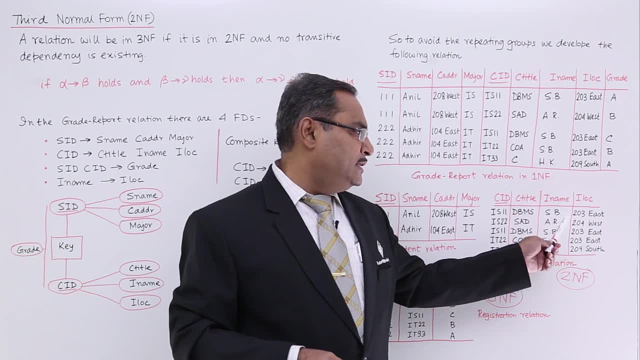 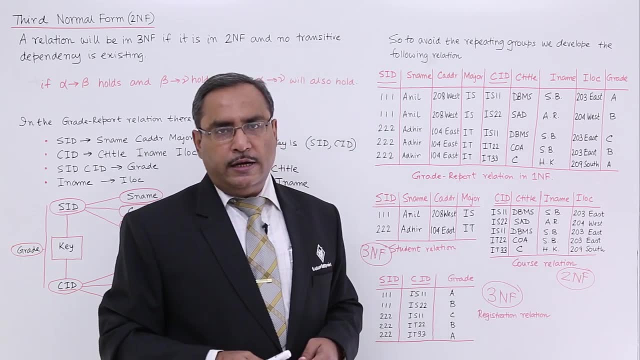 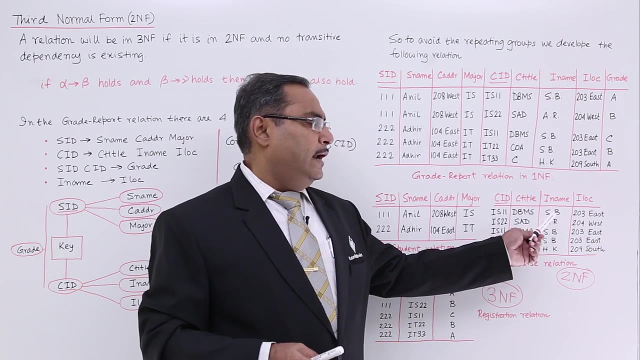 go for the updation anomaly. say hb sb share has changed his address, but his address has been written in multiple locations, so data redundancy is there. so due to the partial updation the database will become inconsistent. so at address: updation of the sb share of sb share will be. 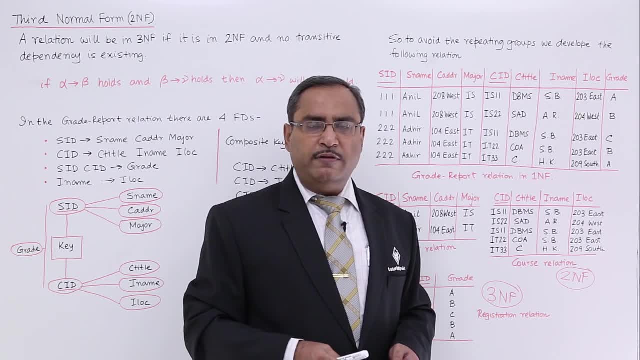 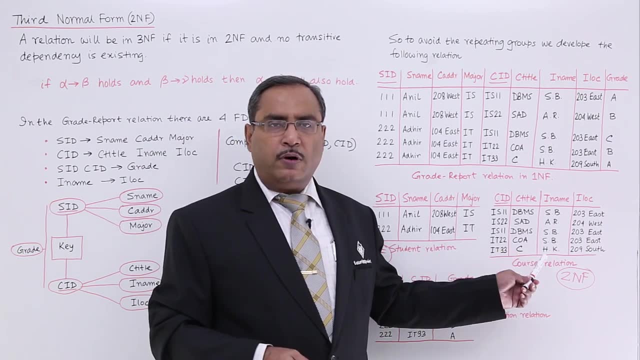 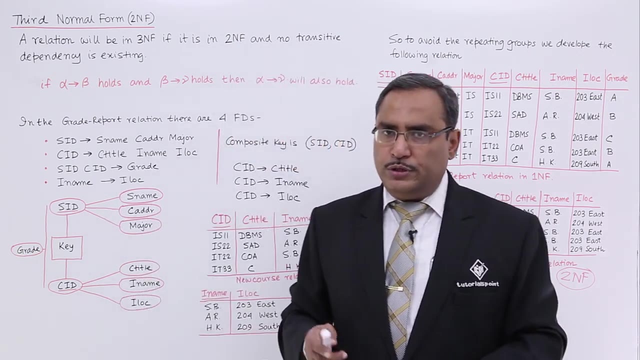 causing partial updation may cause partial updation, leaving the database in some inconsistent state. so that is our updation anomaly. so on this relation i cannot perform insert, delete, update operations. so that is why all the anomalies are there. so let us resolve it. so to resolve this one we can go. 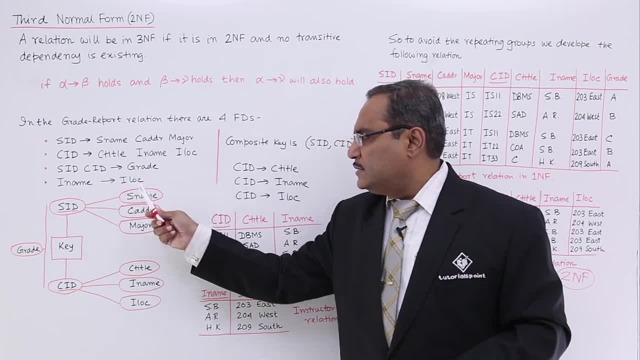 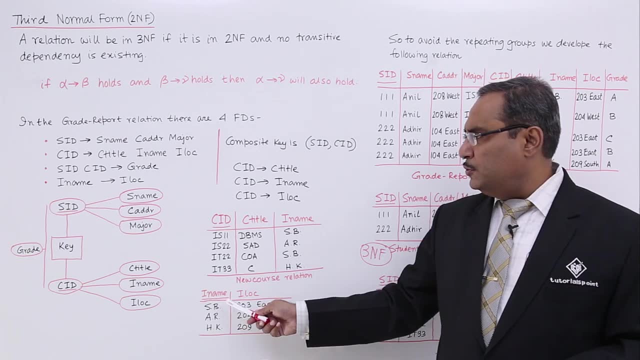 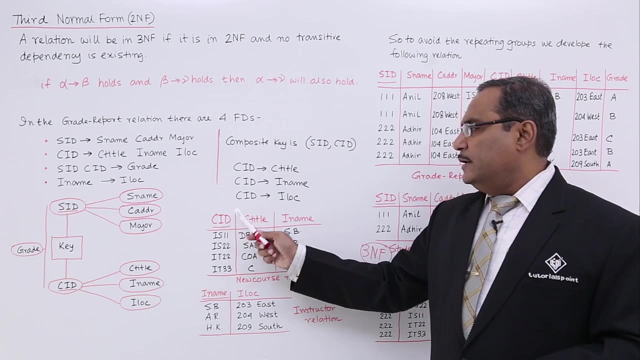 for this. that is, instructor name determines instructors location. so we are making this particular table ready. so here, this is the primary key, this is the prime attribute, and this particular new course relation has been formed, and it has been formed with course id determines course title and instructors name. so this is the relation we have formed. 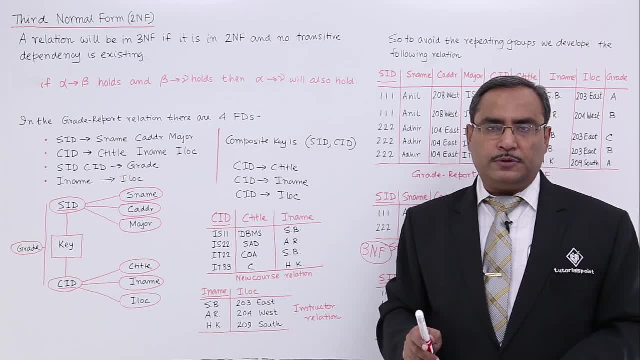 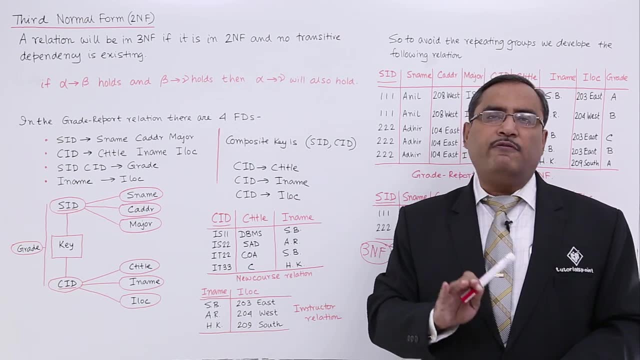 where the course id is the primary key and rest are the non prime attributes. always remember, when you shall split one relation in 3NF you are giving birth to the foreign key because prime attribute in one table it has become a non prime attribute in another table. then 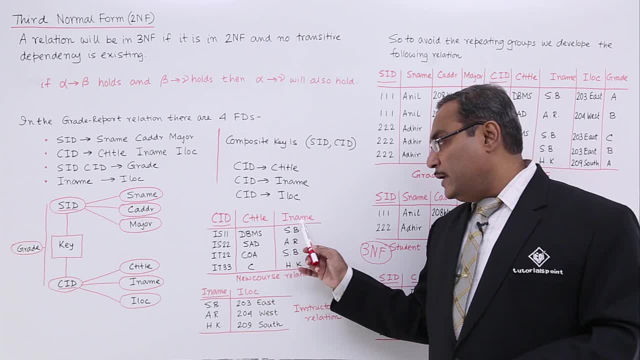 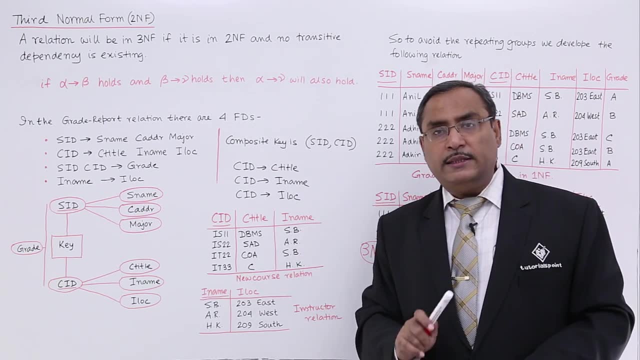 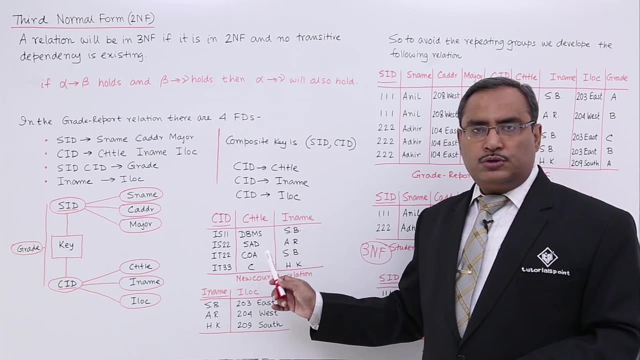 in the second table where it is non-prime. there it is becoming a foreign key. So here this instructor name is becoming a foreign key and whenever there is a foreign key there is a domain constraint. Domain constraint means you cannot assign to any instructor any course, whether this instructor. 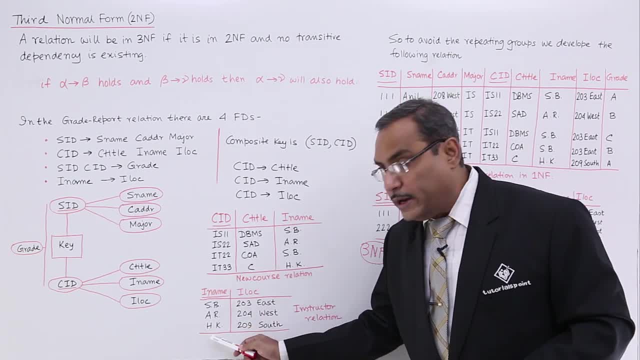 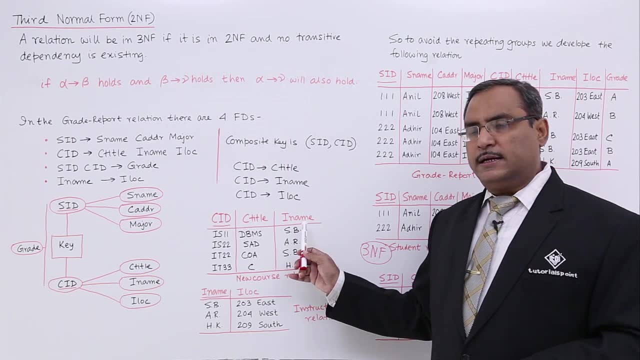 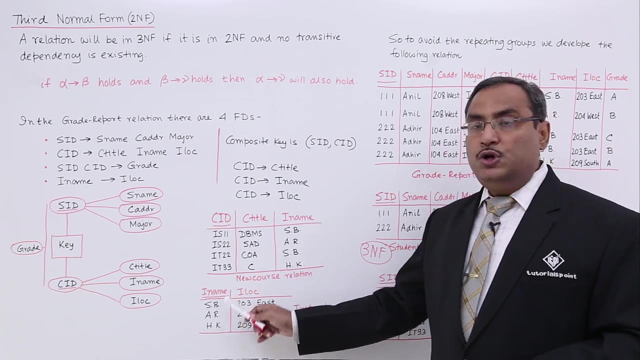 when the instructor name is not belonging to this particular domain. So you cannot write any instructor name under this instructor name column until and unless that instructor name is occurred under the instructor name of this instructor relation. So here we are having this domain constraint. So foreign key is there Always whenever you are splitting one relation using 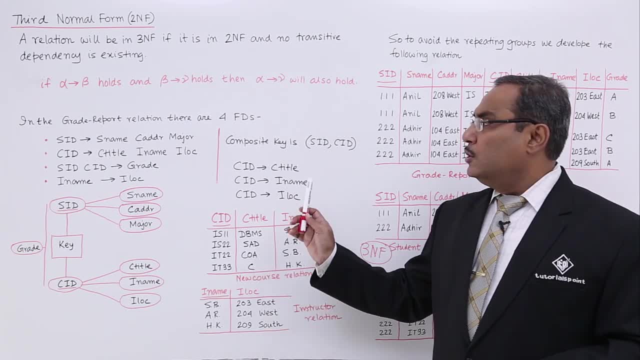 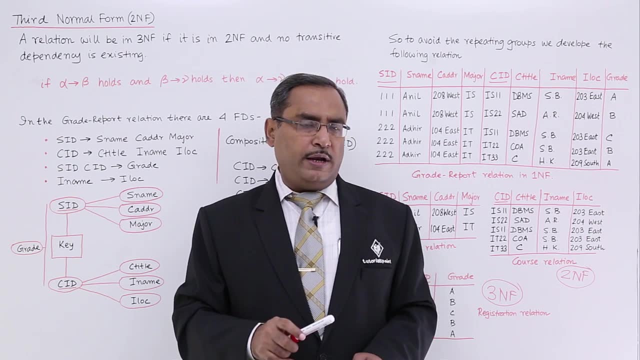 3NF, one foreign key will come into the scene. So here we have discussed what is 3NF, how to bring one relation to the 3NF. If you do not bring the relation in the 3NF, then how the insertion? 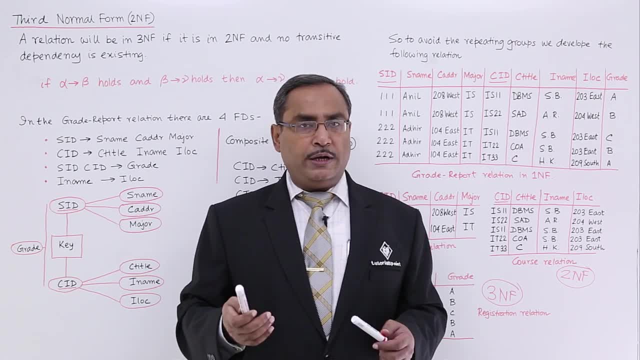